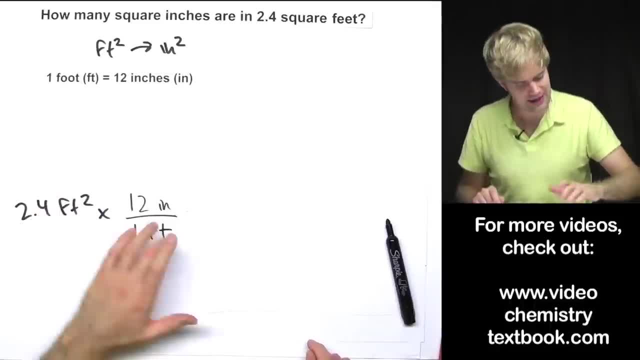 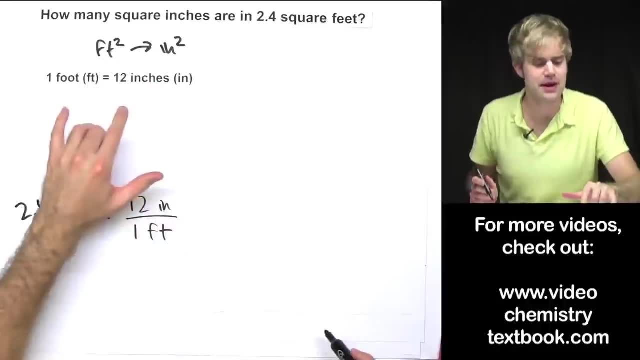 unit down here is just regular feet, So you can't cancel them because they're different units: square feet, regular feet. Subtitles by the Amaraorg community. So we've got to make a relationship that we can then use to build the conversion factor. 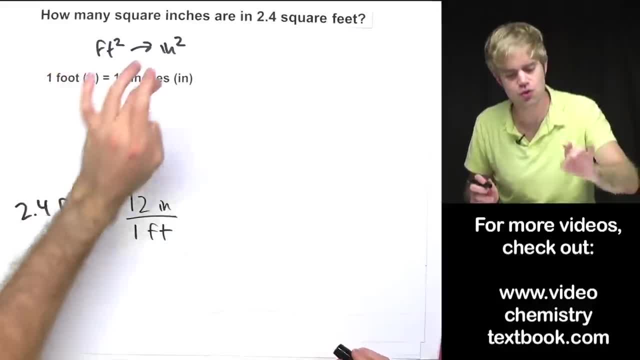 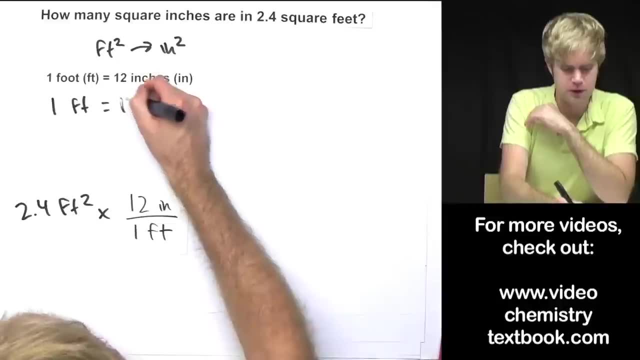 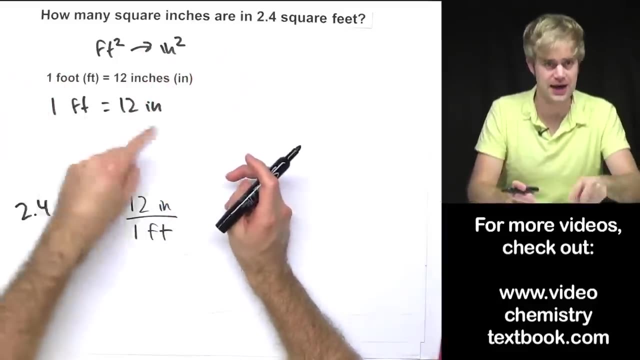 and this relationship has to have square feet and square inches. Here's how we do it. okay, We're going to start by rewriting: one foot equals 12 inches. And now what we're going to do is we're going to square both sides of this. It's fine to square something on. 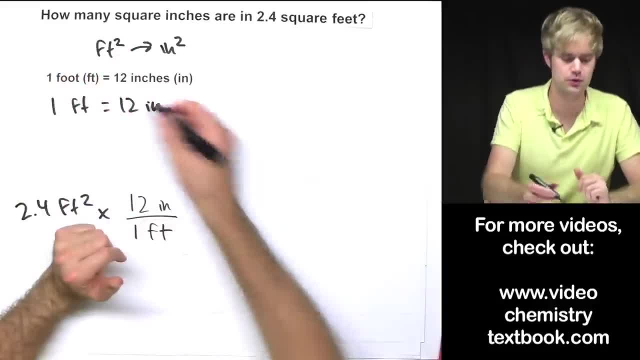 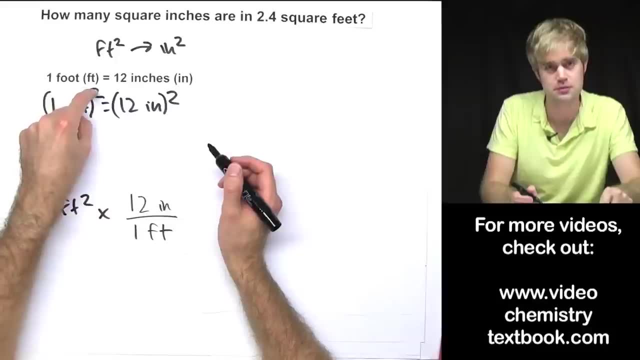 one side of an equal sign, if you square what's on the other side of the equal sign, But if you square what's on the other side of the equal sign. So I'm going to put both of these things in parentheses: squared, squared. Okay, now we have to distribute this exponent. 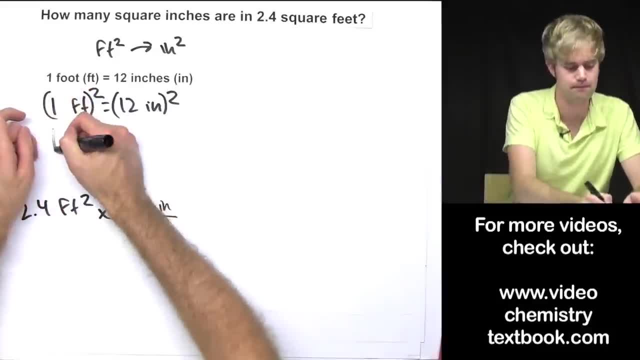 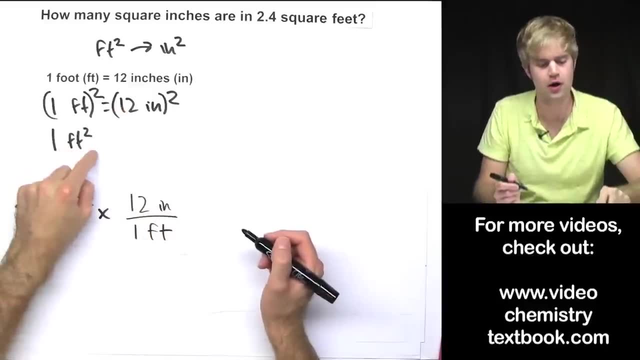 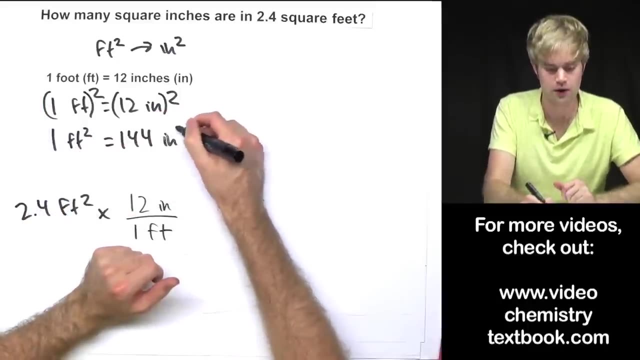 So it's going to be 1 squared equals 1.. And the squared also goes to the feet. So now we've got feet squared, There's our 1 square foot equals 12 squared, That's going to be 144.. And then we've got inches squared. So now we have square inches. Now I can use this. 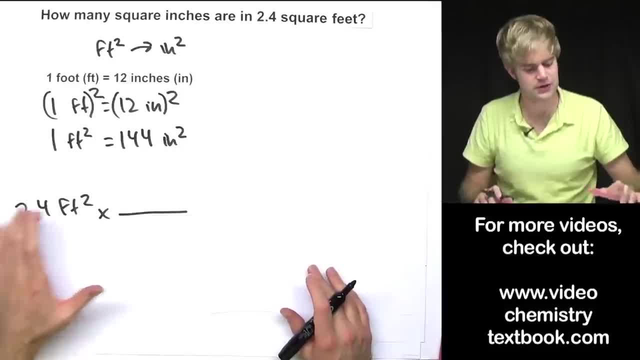 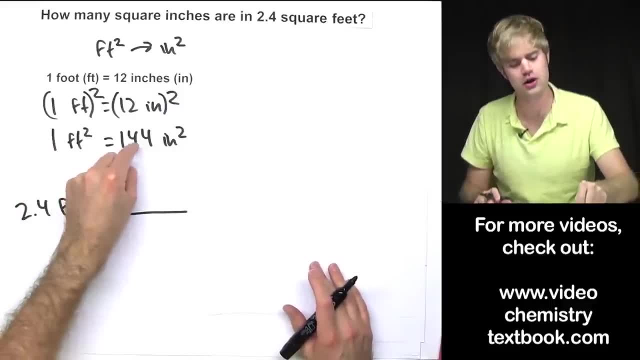 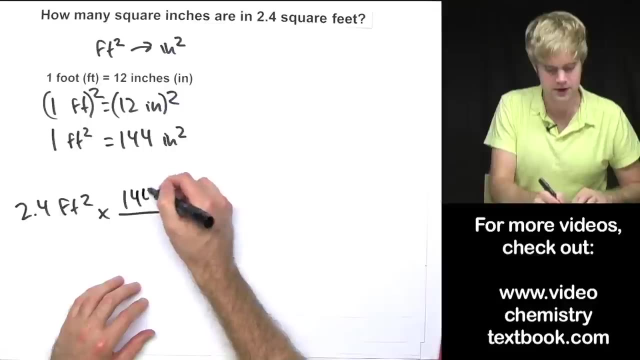 relationship to make a conversion factor that has feet squared or square feet. So this is saying that for every 1 square foot I have, I have 144 square inches. So since I have 2.4 square feet here, I'm going to want to multiply this by the 144 square inches that. 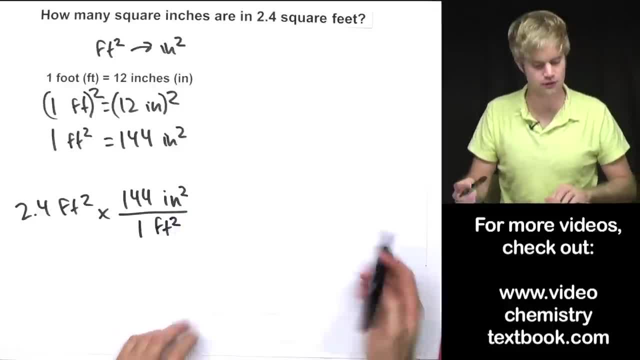 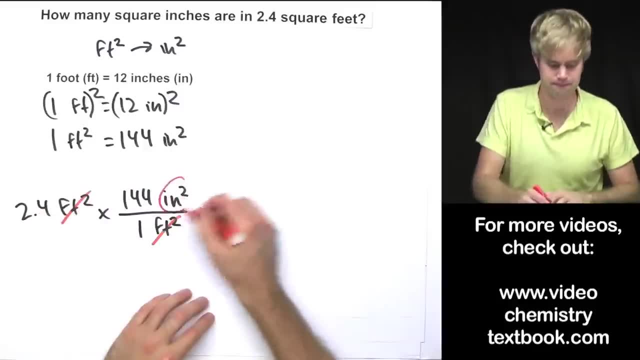 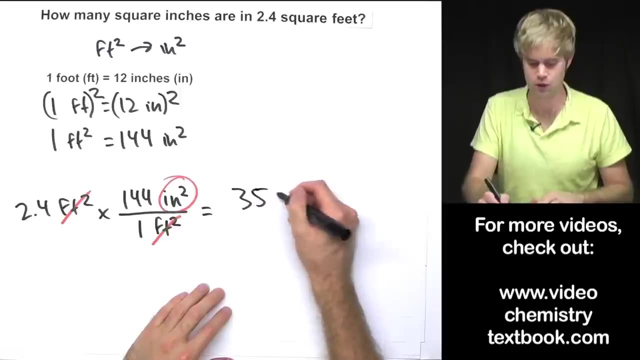 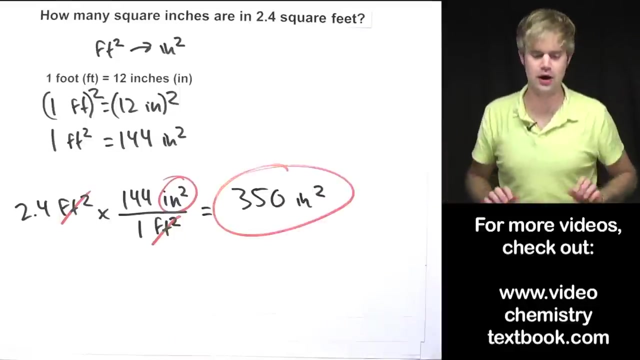 I have in each of my 1 square feet. Now I have square feet up here and square feet down there, so they'll cancel out. That leaves me with units of square inches, And I'll do 2.4 times 144 divided by 1, rounded to 2 significant figures, equals 350 square inches. Now let's. 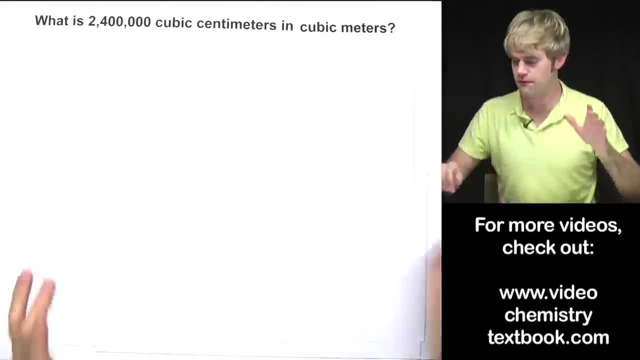 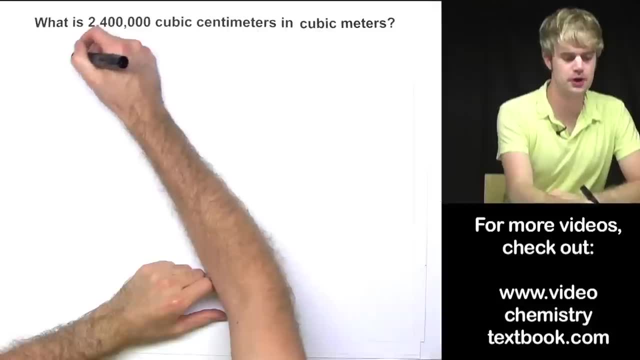 look at units of volume. What is 2,400,000 cubic centimeters in cubic meters? The answer might surprise you. So we're going from centimeters cubed to 3,000 cubic meters. So we're going from centimeters. 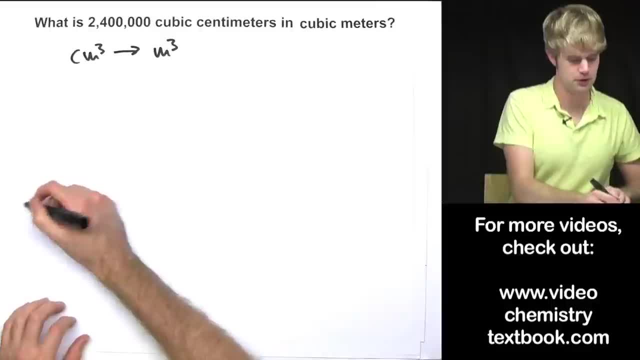 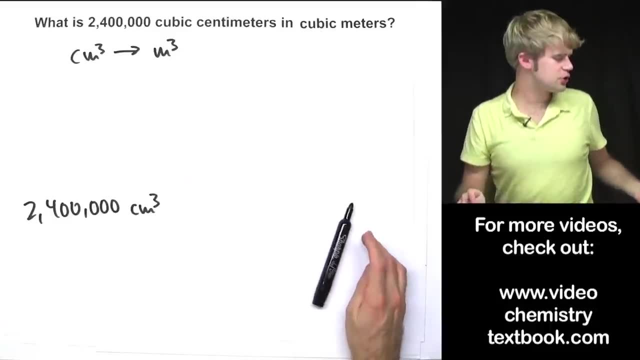 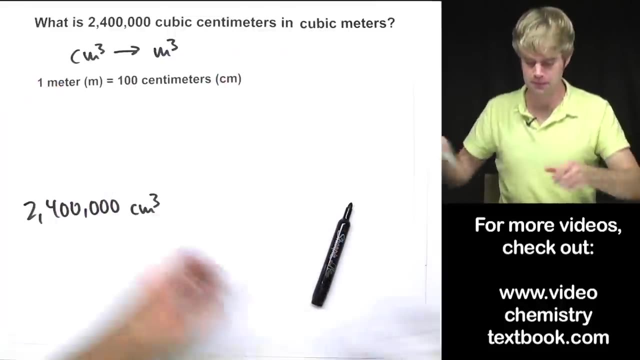 cubed to 3,000 cubic meters. So we're going from centimeters cubed to 3,000 cubic meters And we're starting with 2,400,000 cubic centimeters. The relationship between meters and centimeters is that there are 100 centimeters in 1 meter. But, as we saw before, don't mess up and think. 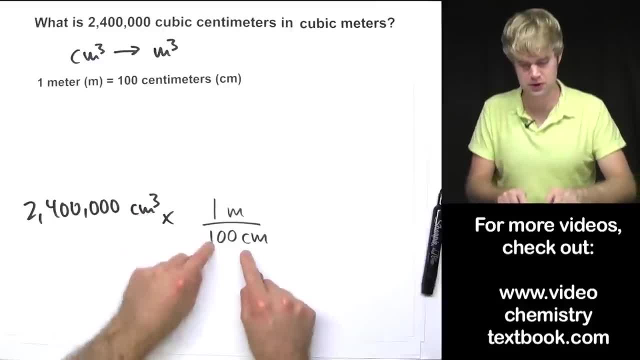 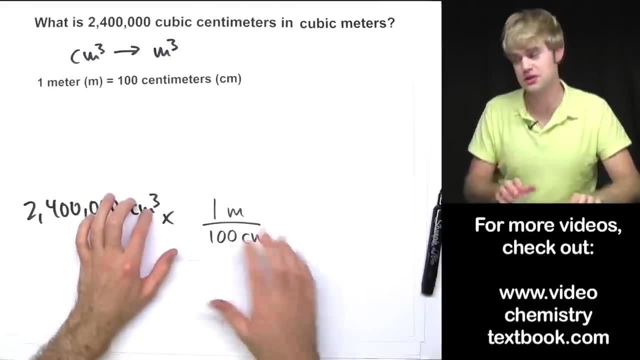 that you can write a conversion factor to get rid of cubic centimeters by putting something like this with 100 centimeters on the bottom: No, because these are regular centimeters, they're not cubic centimeters. So to get this into a relationship that will give us cubic, 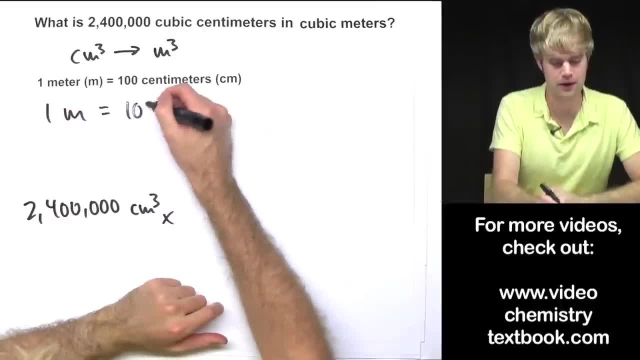 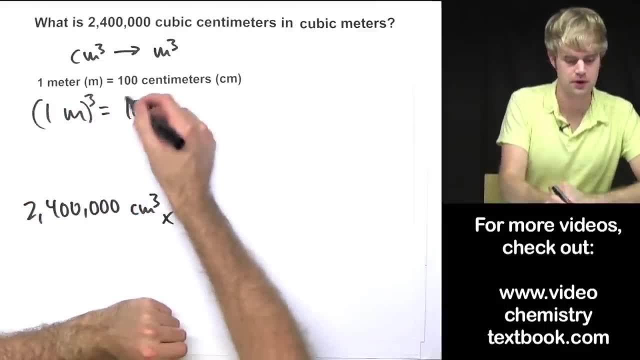 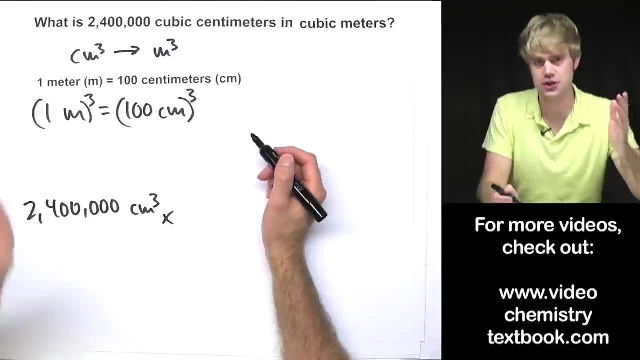 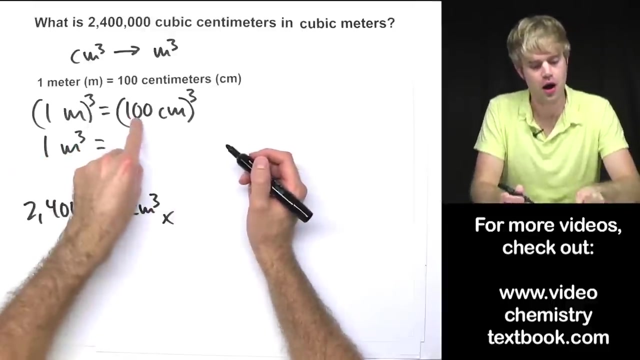 centimeters. we're going to rewrite: 1 meter equals 100 centimeters. And now I'm going to cube both sides of the equation, This to the third and this to the third. Distribute this Now, 1 to the third just equals 1.. Meters to the third gives us 1 cubic meter Now. 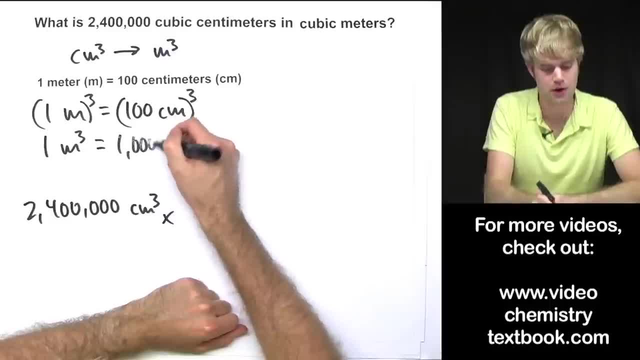 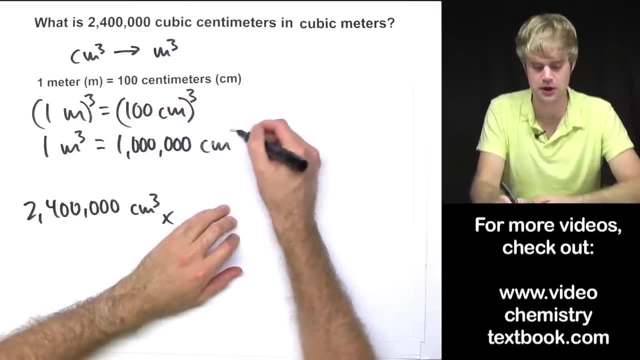 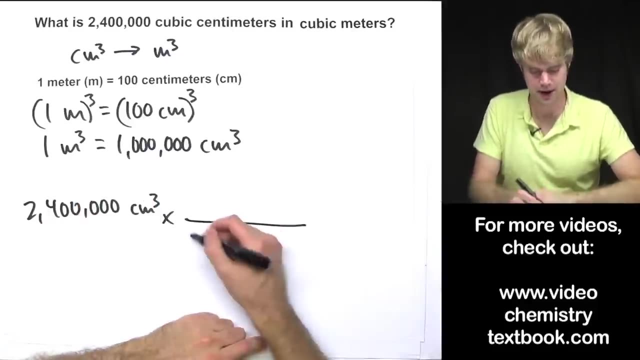 100 cubed is 1 million right 100 times 100 times 100 and now the cube distributed onto centimeters gives cubic centimeters. So the conversion factor now is going to put cubic centimeters on the bottom. so I'm going. 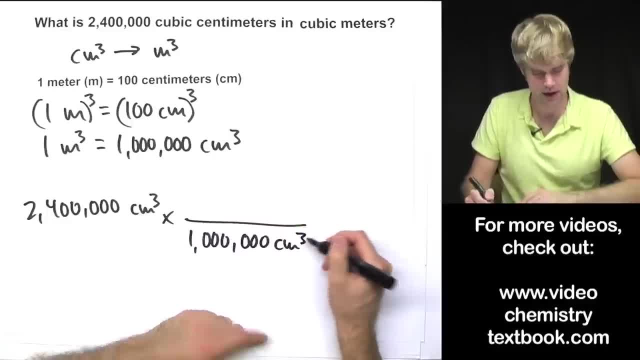 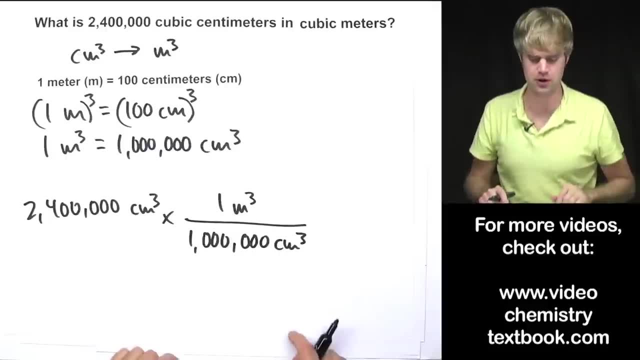 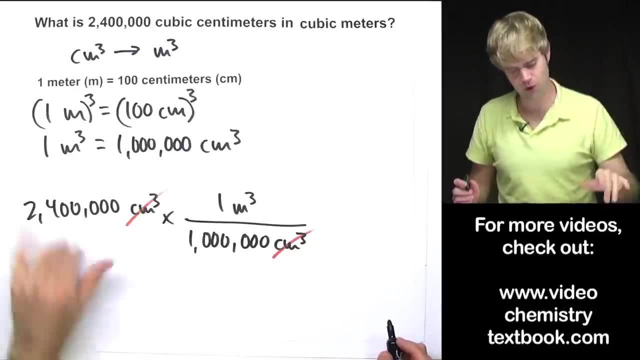 to have a million cubic centimeters and I'm going to have one square meter on the top, just telling us that for every one square meter we have, we have a million cubic centimeters. Cubic centimeters on the top, on the bottom, 2,400,000 times 1 divided by a million is. 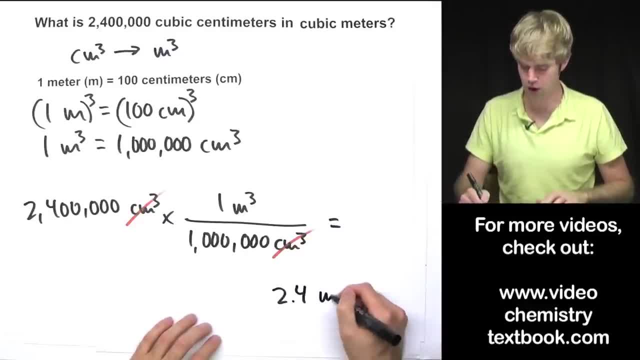 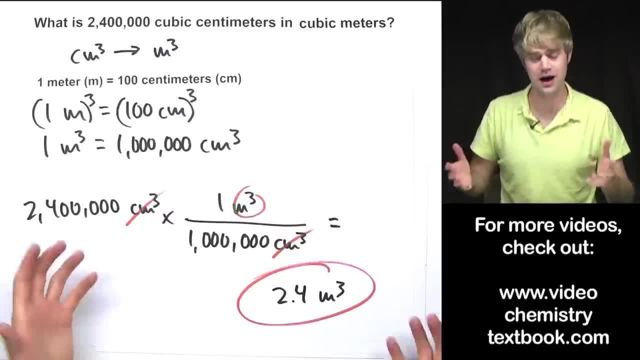 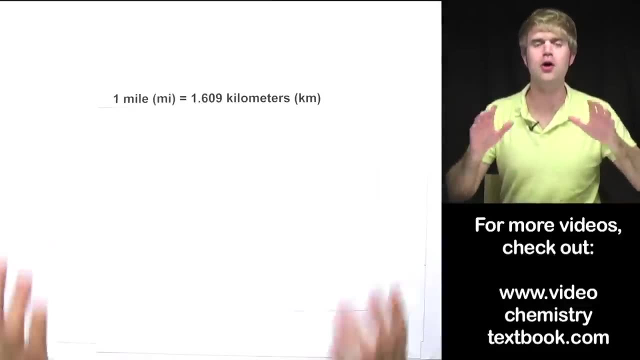 going to give us 2.4 cubic meters, So a whole bunch of cubic centimeters are not that much in cubic meters. So you can use this strategy. You can use this strategy of squaring, cubing both sides of a relationship to come up with 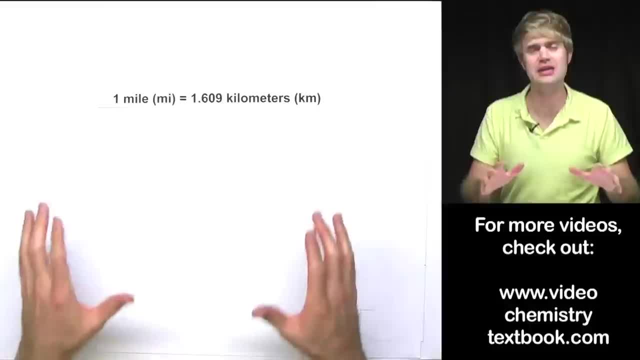 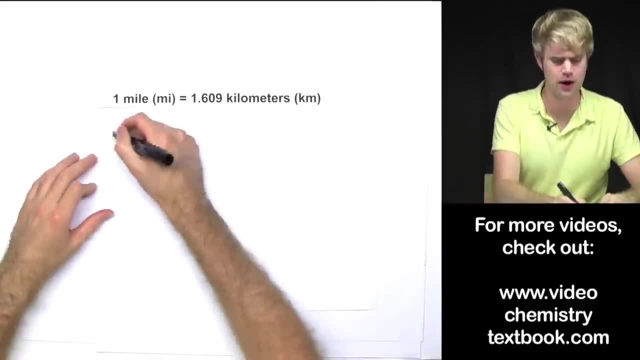 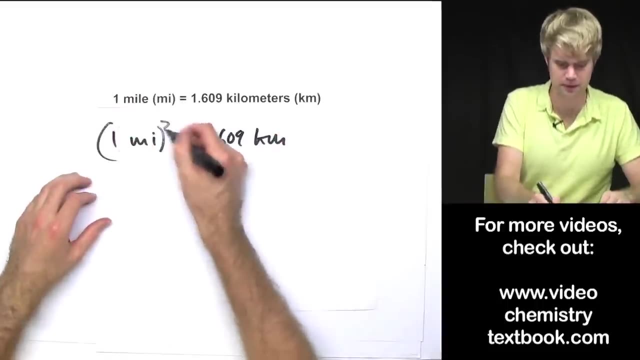 conversion factors that you can use to convert between any squared units of area or cubed units of volume. So, just as one last example, if I wanted to convert between, say, square miles and square kilometers, I just take this relationship and I'd square both sides, giving me one square.